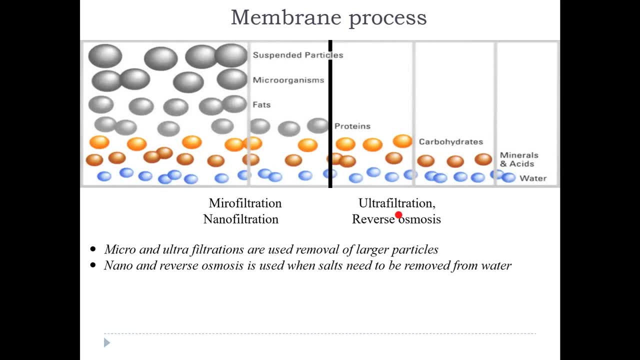 In this video we are going to study about some membrane processes, especially reverse osmosis and ultra filtration. These are very common techniques that we use in our home filters. Okay, you must have seen this Hema Malini ad about RO and everything. keln filters right. 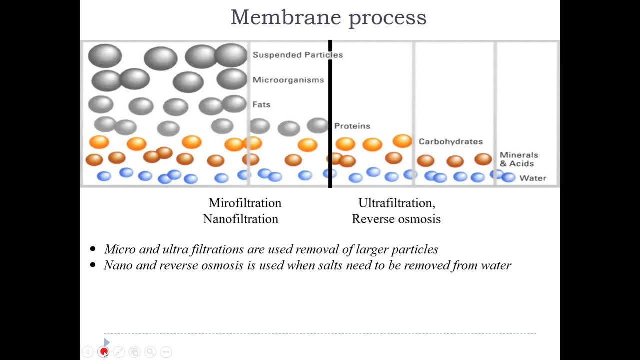 Okay, so that is nothing but filtration techniques, that is, membrane processes. What exactly these processes do? we have a small, we have a semi permeable membrane. it's kind of you know filtration. So depending upon the size of the pose, different particles can be filtered. and 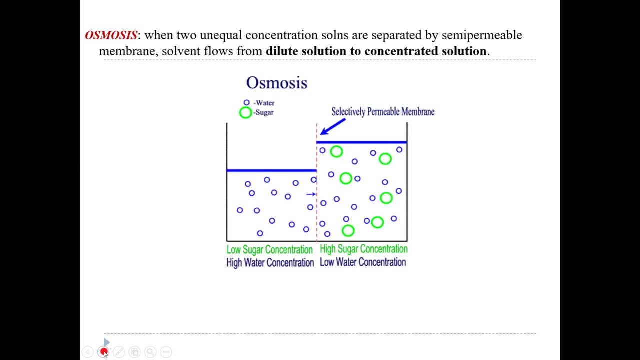 removed from the water. So the first one is reverse osmosis. Before studying reverse osmosis, you should know what is osmosis. Osmosis means what? Two solutions? when they are separated by a semi permeable membrane, the solvent flows from dilute solution to concentrated solution. 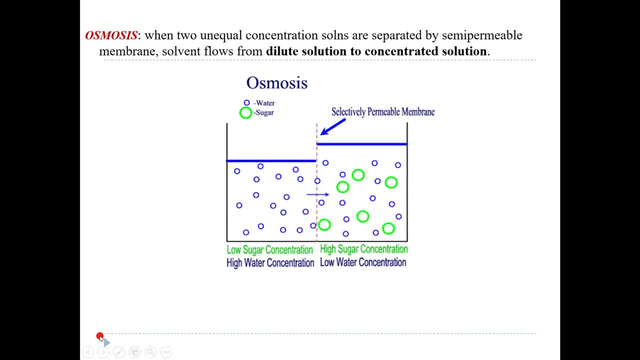 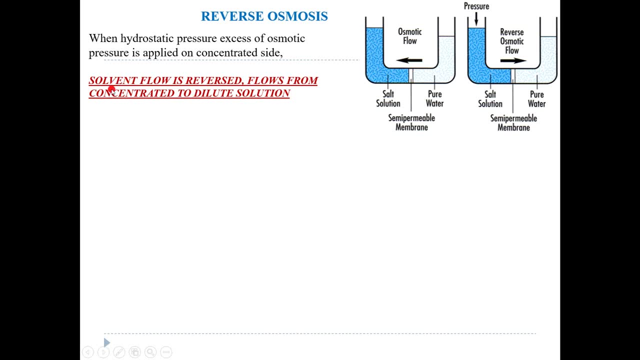 So this is a normal osmosis process? Okay, And reverse osmosis is exactly opposite. Reverse of osmosis, It is the process where a solution flows from higher concentration to lower concentration, concentrated solution to dilute solution. And how does this happen? Because of 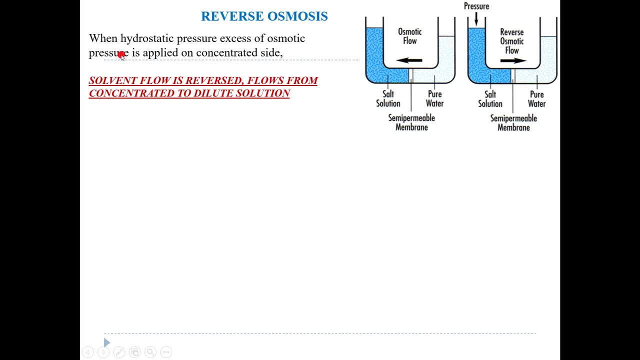 hydrostatic pressure is in excess of osmotic pressure, It is applied on the concentrated side. So when hydrostatic pressure excess of osmotic pressure is applied, the solvent flows from concentrated to dilute solution And it's kind of you know. 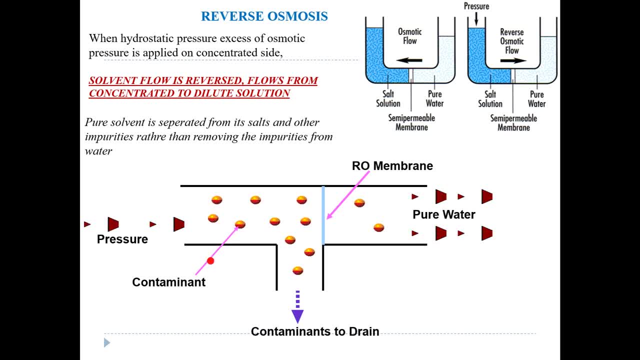 it's like when you apply this pressure, you can see the pressure over here. It is like water is getting separated and the contaminants are staying on the other side of the permeable membrane. So pure solvent is separated from its salts and other impurities rather than 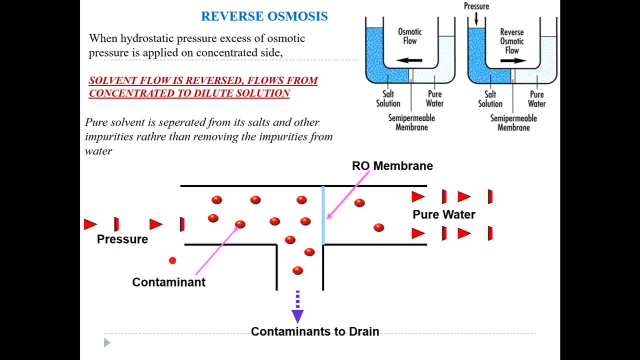 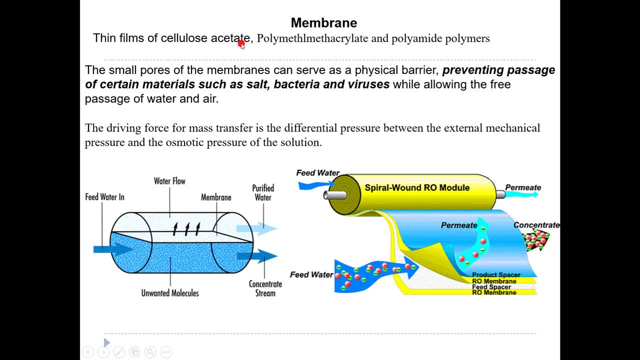 impurity, removing the impurities from the water. Exactly opposite. So we are separating water, not the impurities. Now this membrane: it's a semi permeable membrane made up of cellulose acetate, polymethamethacrylate, polyamide polymers, and they have small pores which 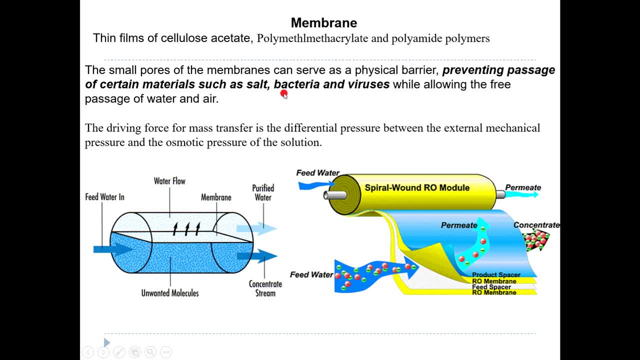 prevent the passage of certain materials like, say, salt, bacteria, viruses. And what does our water contain? These are the most major things that our water contains. So all these are, you know, separated, they are retained by the membrane And, of course, all these, 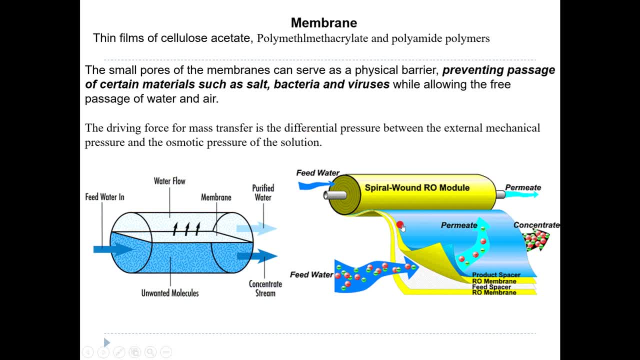 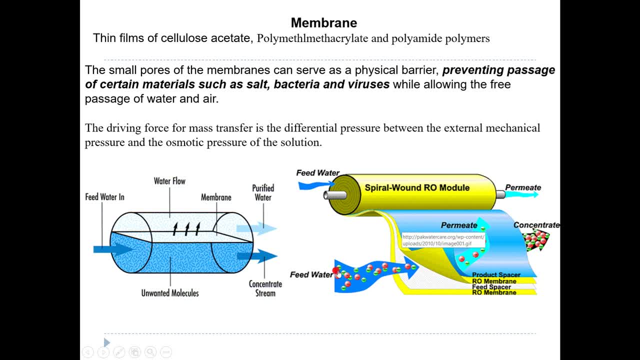 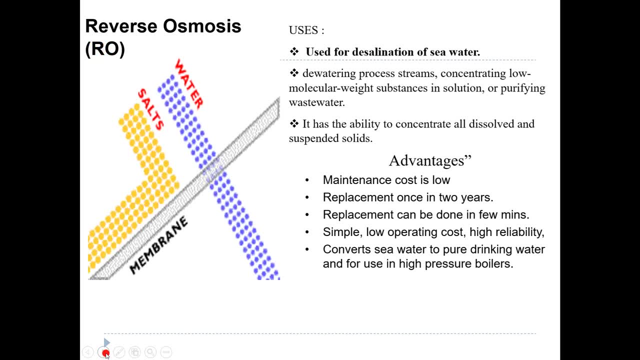 You can see this: how this membrane is made of and how it is wound off and kept in that cartridge. So what is the use of reverse osmosis? The most important use of reverse osmosis is desalination of seawater. Your seawater contains so many salts, bacteria, viruses. 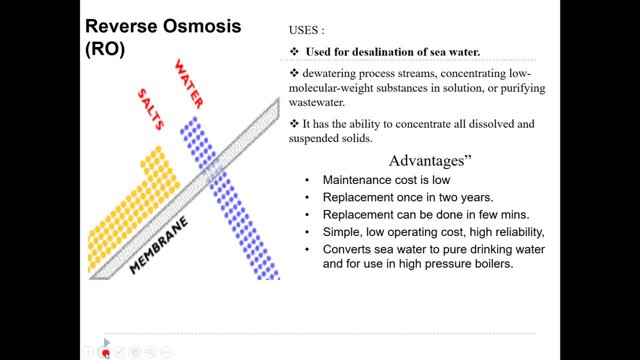 all these can be separated by reverse osmosis. It's, like you know, converting seawater into fresh water, saline water, capable of drinking. Okay, Apart from that, you can do concentration of low molecular weight substances in the solution, because you are removing water, So you're concentrating the solution. purify. 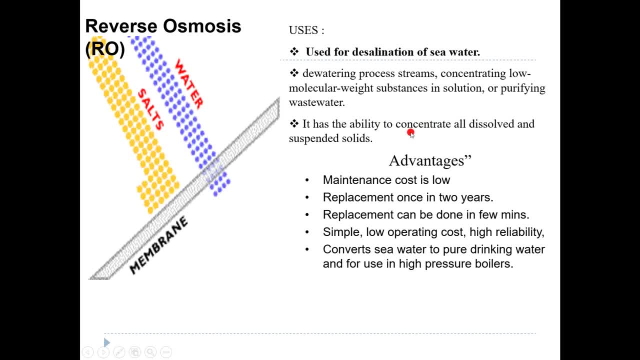 the wastewater. Okay, So it is. it has the ability to concentrate all dissolved and suspended solids, because you are removing water from these solids, Right, And what are the advantages? Like you know, this RO technique is easily available in our filter, So its maintenance. 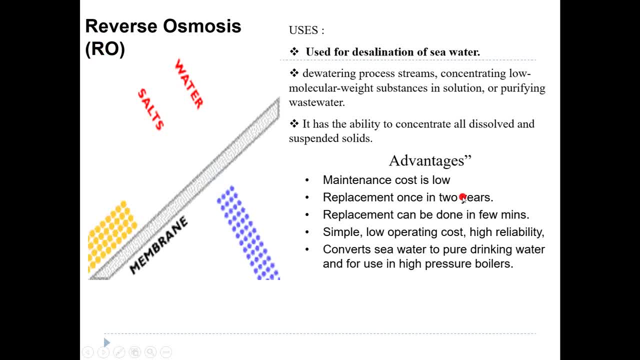 cost is low. You just have to replace that membrane. in one or two years It can. this replacement can be done in few minutes. low operating cost, high reliability. convert seawater into pure drinking water. That water can be used for high pressure boilers, Remember. 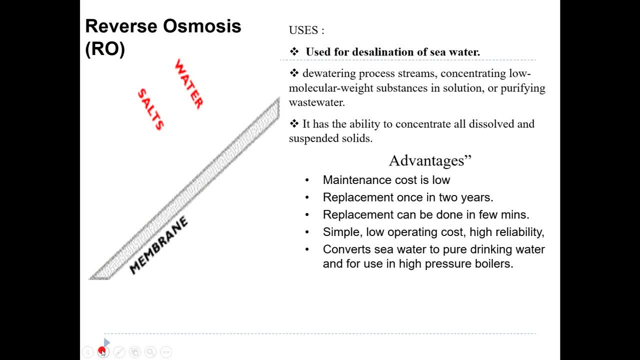 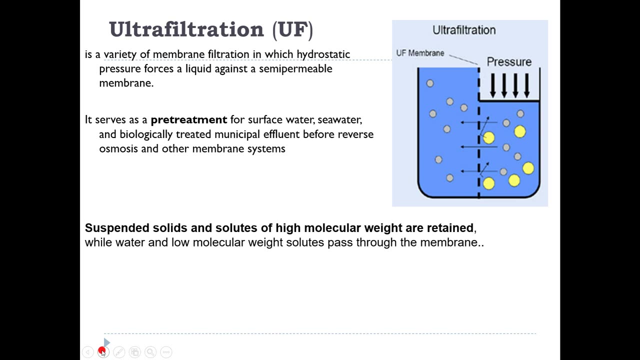 boilers. they have this sludge and scales are formed. So the normal water is not good for that, or hard water is not good for that. So for such boilers where a lot of water is used, you can use this reverse osmosis process and use this water for boilers- The next type. 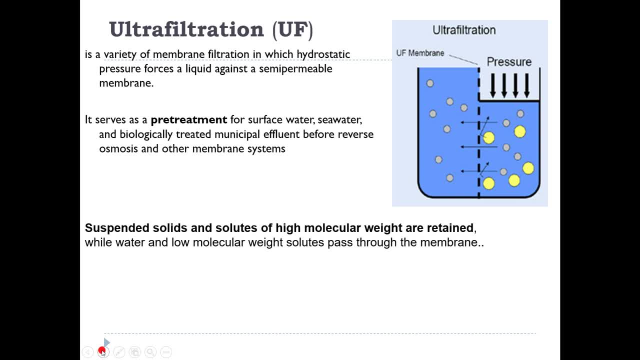 of process is ultrafiltration, Kind of pre-treatment to reverse osmosis? Uh, it is a variety of membrane filtration in which hydrostatic pressure forces the liquid against a semi-permeable membrane- similar type of technique to reverse osmosis. It serves as a pre-treatment for surface water, seawater. 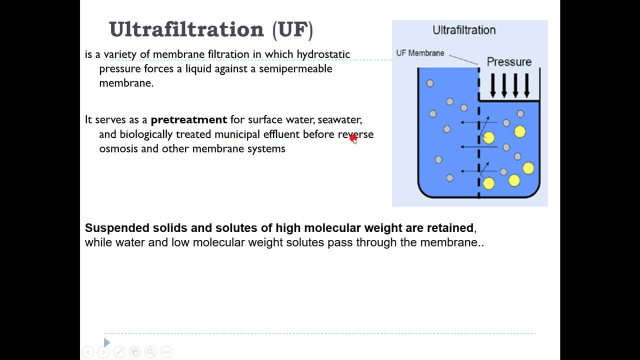 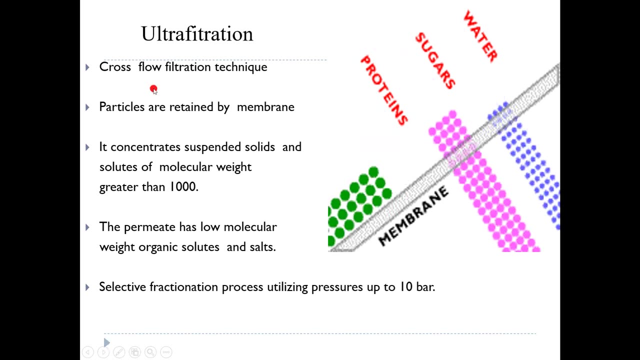 and biologically treated municipal effluent before reverse osmosis: Okay, So suspended solids and solutes of higher molecular weights are retained and only water and low molecular weight solutes Allowed to pass through this membrane. It's a cross flow tracking. Particles are retained. 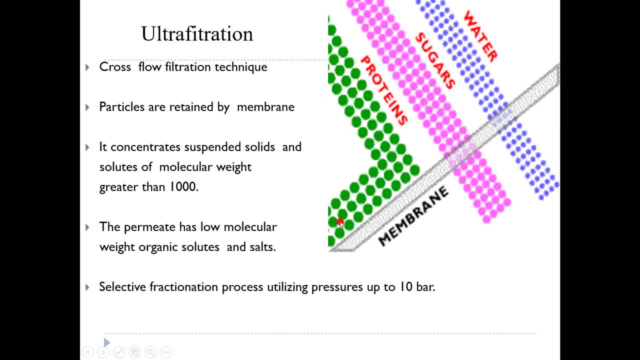 by the membrane. As you can see, the protein particles are retained by the membrane and the small particles like salt, sugar and water are allowed to pass through the membrane. It concentrates suspended solids and solutes of molecular weight greater than thousands, So higher molecular weight compounds are retained. They can be concentrated. Permeate has low. 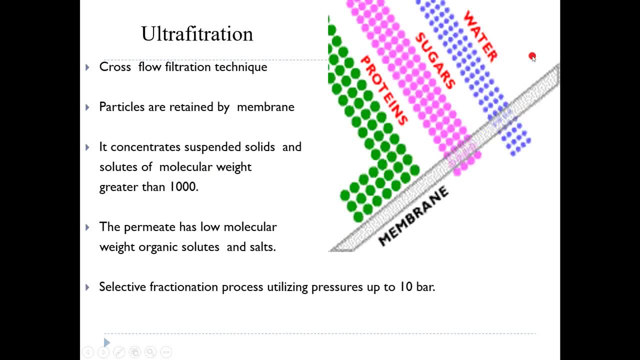 molecular weight. So whatever filtrate of permeate, the permeate means the solution that is coming out through the membrane. So the permeate has low molecular weight. So this is the permeate. It contains no molecular weight substances like salt or sugar, organic. 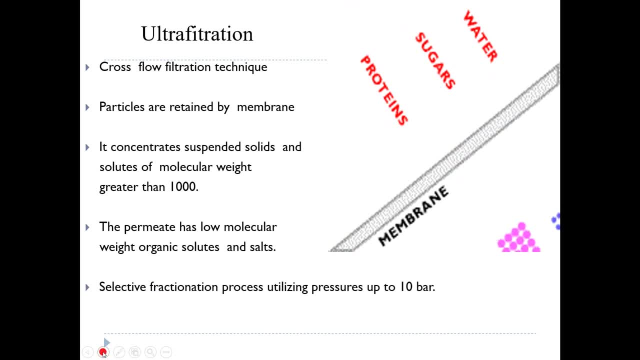 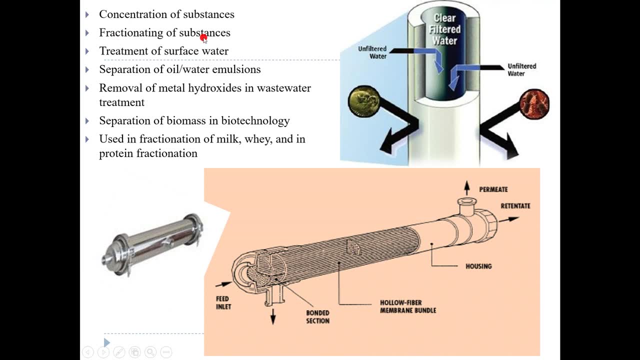 compounds and the pressure is used up to 10 bars. Now, this is. these are some of the advantages and uses. it is used for the concentration of the substances, fractionating of the substances, separating towards more solids, treatment of sulphur sorry surface water. separation of oil and water. oil and water can be separated. 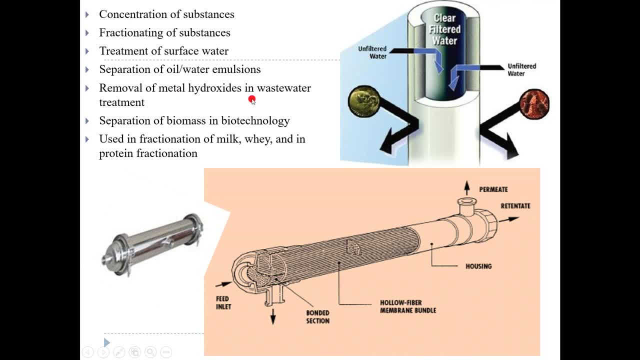 Oil is retained and water is allowed to pass. group surface water. Kidney is separated from retained water is allowed to pass. metal hydroxides can be removed. biomass separation of biomass. in biotechnology it is used in fractionation of milk. if you can, if you have seen that proteins are. 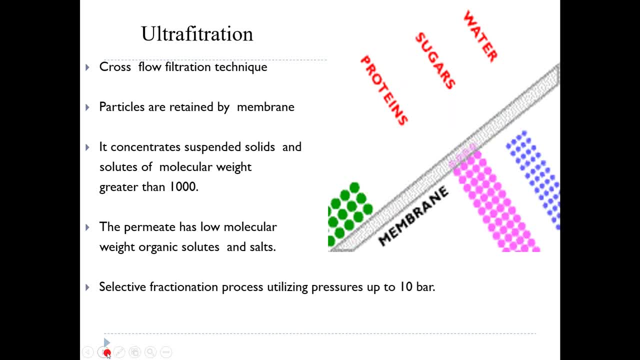 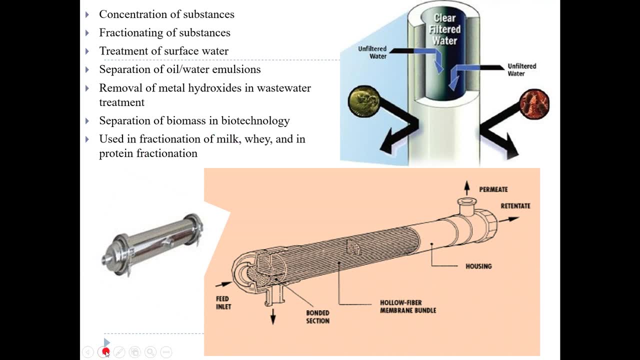 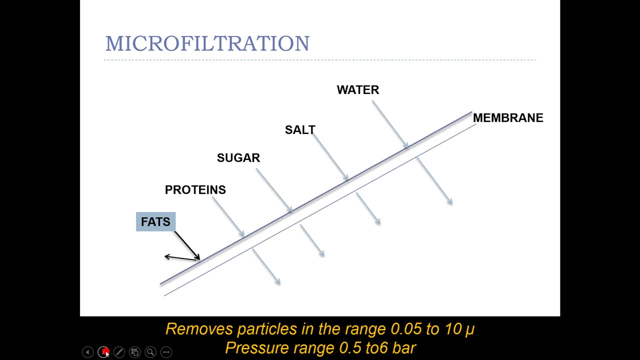 separated, no, so protein concentration can take place. so you are separating water and other salts, so protein concentration can take place over here. so it is used in fractionation of milk way okay. apart from that, apart from these two processes, there are other membrane processes. depending upon the size of the pore, certain materials can pass through it and certain 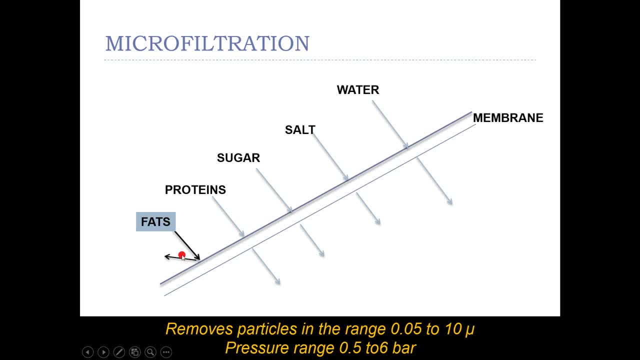 materials are retained, for example micro filtration. the pore size is comparatively larger, so only fats are retained, whereas protein, sugar, salts, water are allowed to pass through it, and so this is the range of the particles which can, which can be removed. then you have ultra filtration, see the 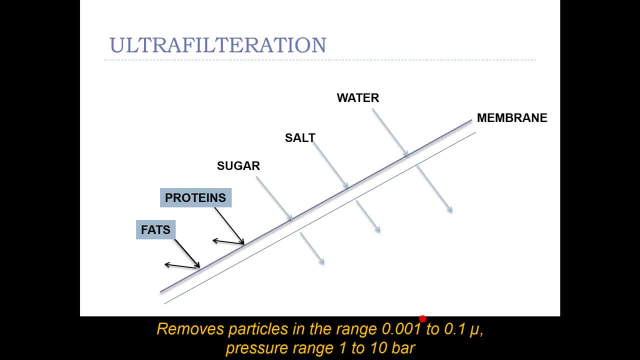 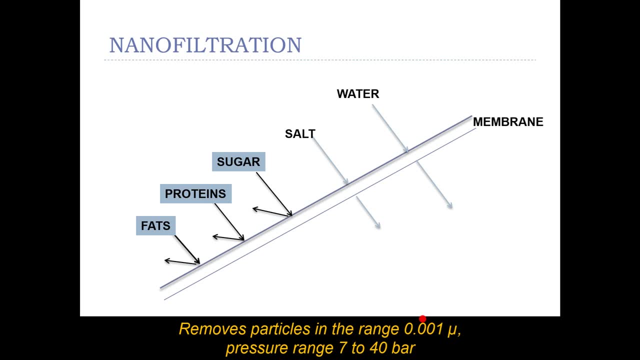 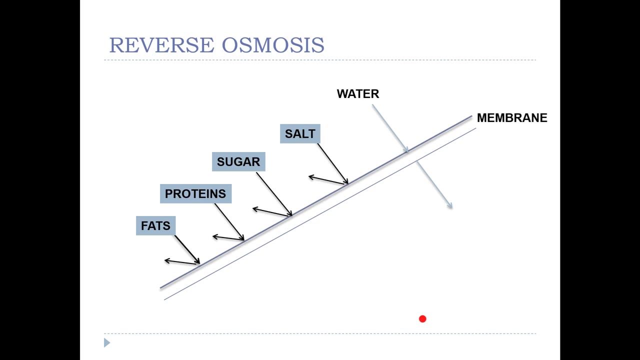 difference. your micro filtration separates out the fats. ultra filtration separates out the proteins. my nano filtration separates out sugar, and i guess you must have guessed it, this is reverse osmosis, which has separated the salt as well. so these were some of the membrane processes, which is enough for you as far as your syllabus is concerned. 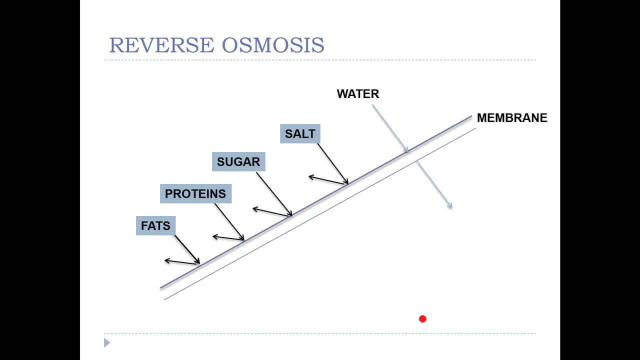 do watch the next other videos on activated sludge and microorganism treatments. thank you.